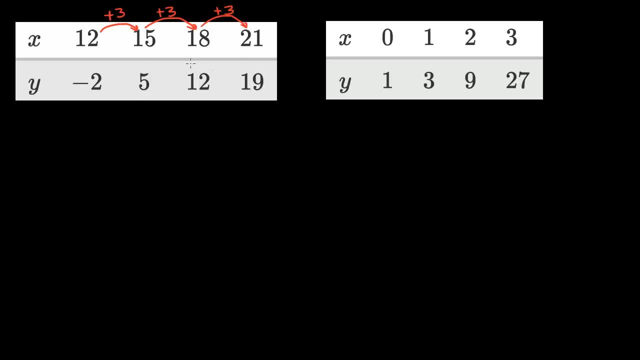 Or is there a constant ratio between successive terms when you increase x by a constant amount, in which case we would be dealing with an exponential relationship? So let's see Here we're going from negative two to five, so we are adding seven. 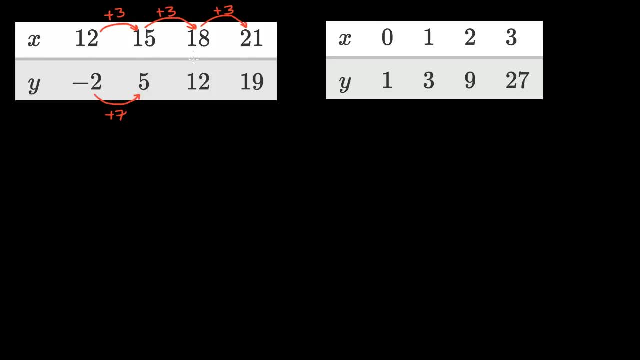 When x increases by three, y increases by seven. When x is increasing by three, y increases by seven again. When x increases by three, y increases by seven again. So here it is clearly a linear relationship, Linear relationship, In fact you can even relationship. 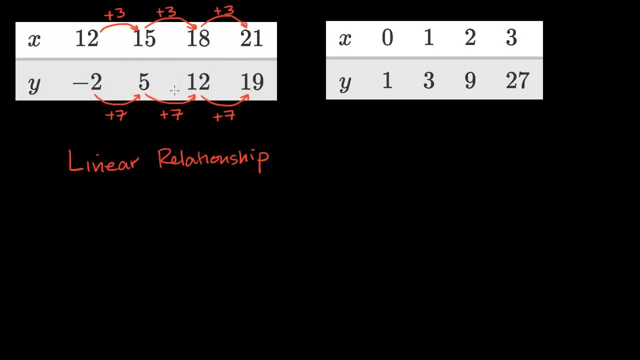 You could even plot this on a line. if you assume that these are samples on a line. You could think even about the slope of that line. For a change in x, for a given change in x, the change in y is always constant. 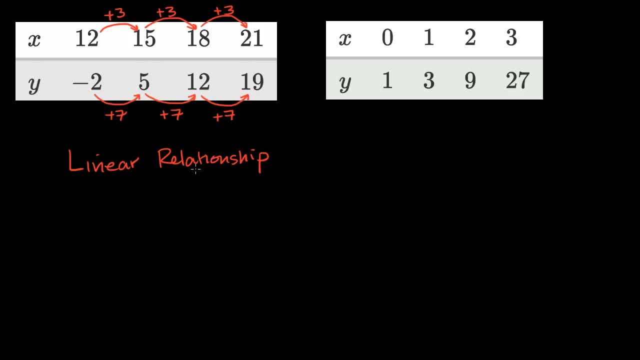 When our change in x is three, our change in y is always seven. So this is clearly a linear relationship. Now let's look at this one. Let's see, Looks like our x's are changing by one each time. So plus one. 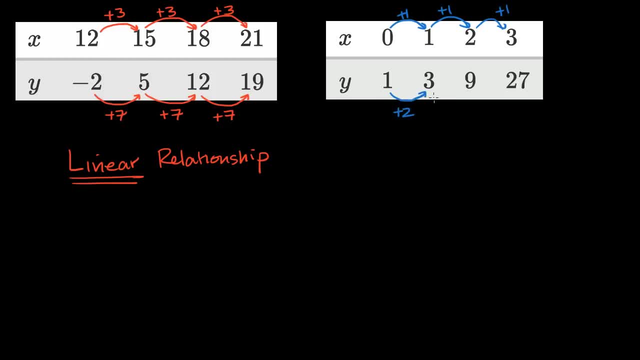 Now, what are y's changing by? Here it changes by two, then it changes by six. All right, it's clearly not linear. Then it changes by 18.. Clearly not a linear relationship. If this was linear, this would be the same amount. 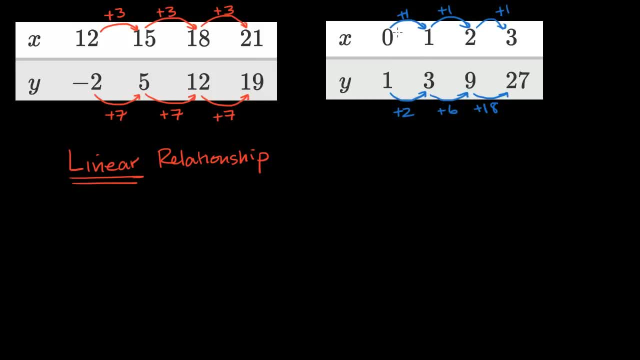 same deltas, same change in y for every time, because we have the same change in x. So let's test to see if it's exponential, If it's an exponential for each of these constant changes in x's when we increase x by one every time. 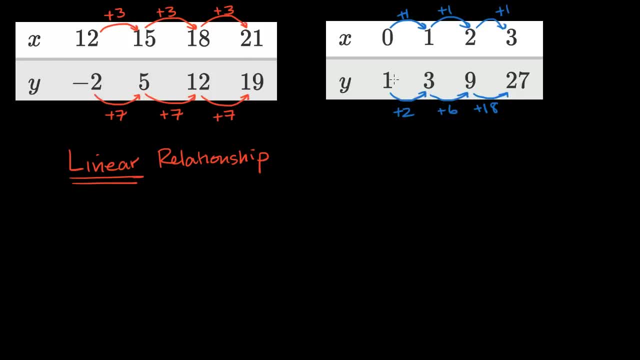 our ratio of successive y should be the same. Or another way to think about it is: what are we multiplying y by? So, to go from one to three, you multiply, you multiply by three. To go from three to nine, you multiply by three. 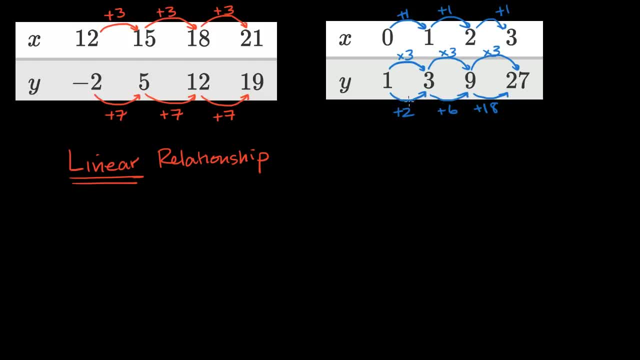 To go from nine to 27,. you multiply by three. So in a situation where every time you increase x by a fixed amount- in this case one- and the corresponding y's get multiplied by some fixed amount, then you are dealing with an exponential relationship. 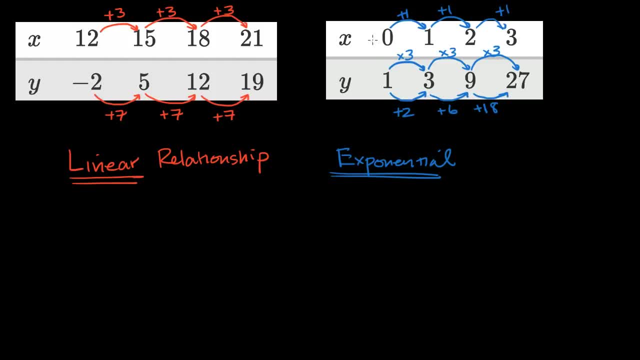 Exponential, exponential relationship right over here.